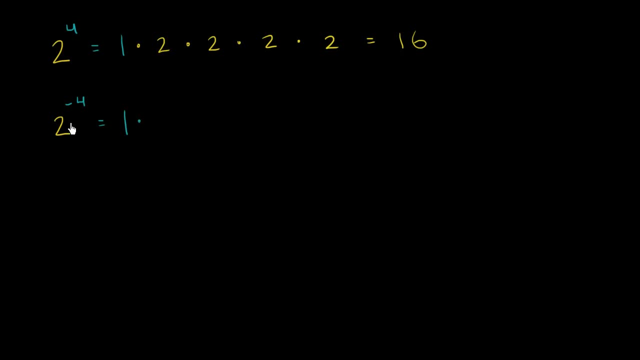 So this could be viewed as 1 times, And we're going to divide by 2, four times. Well, dividing by 2 is the same thing as multiplying by 1 half, So we could say that this is 1 times, 1 half times. 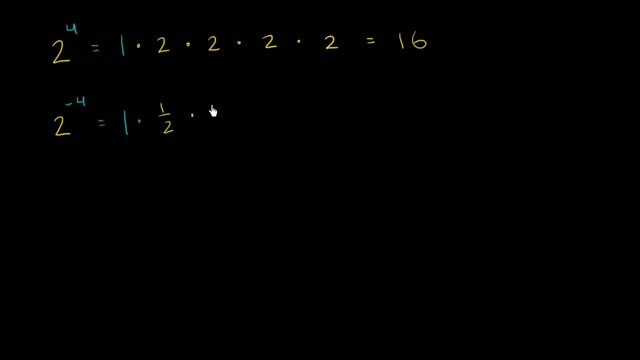 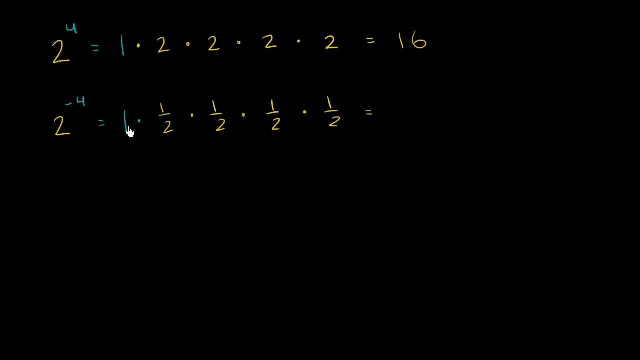 And in this situation, this would get you 1 half. Well, 1 times 1 half is just 1 half Times. 1 half is 1 fourth Times. 1 half is 1 eighth Times. 1 half is 1 over 16.. 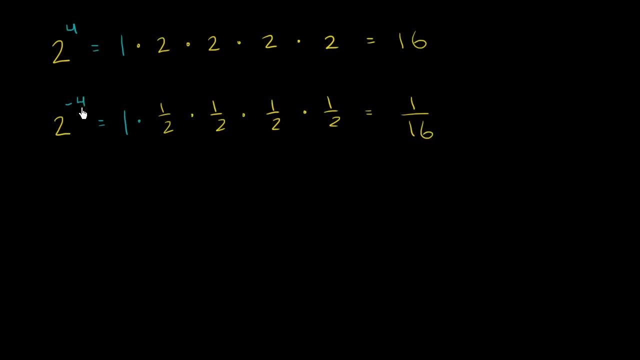 And so you probably see the relationship here. This is essentially: you're starting with the 1, dividing by 2 four times. You could also say that 2 to the negative 4 is the same thing as 1 over 2 to the fourth power. 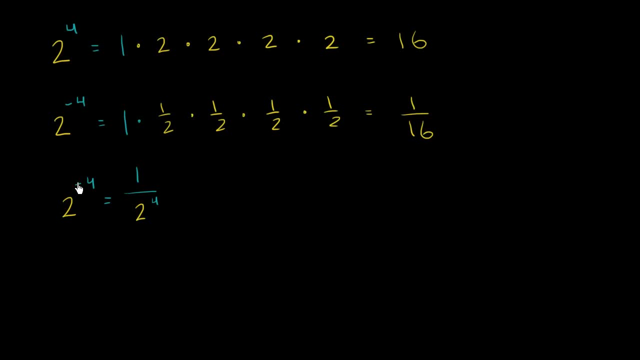 Let me color code it nicely so you realize what the negative is doing. So this negative right over here. let me do that in a better color. I'll do it in magenta, something that jumps out. So this negative right over here. 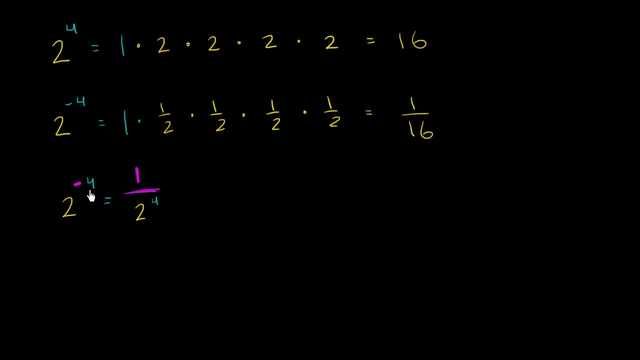 this is what's causing us to go 1 over. So 2 to the negative 4 is the same thing, based on the way we've defined it just up right here as 1 over, or the reciprocal of 2 to the fourth. 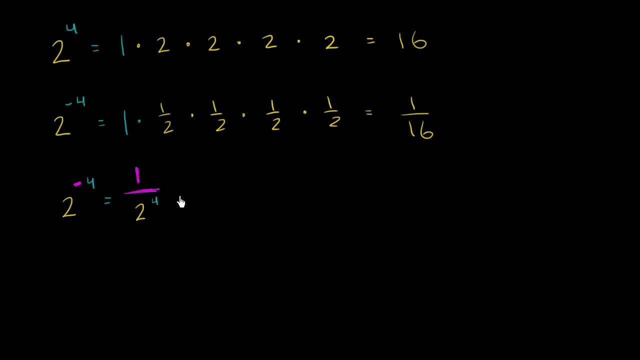 or 1 over 2 to the fourth, And so you could view this as being 1 over 2 times, so 2 times 2 times 2 times 2.. If you just do 2 to the fourth as taking four twos, 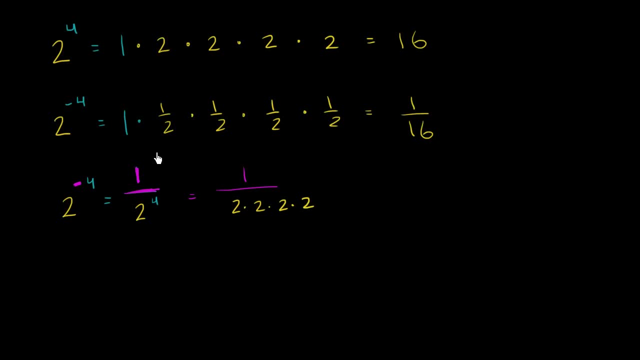 and multiplying them. Or if you use this idea right over here, you could view it as starting with the 1 and multiplying it by 2- four times. Either way, you are going to get 1 over 16.. So let's do a few more examples of this. 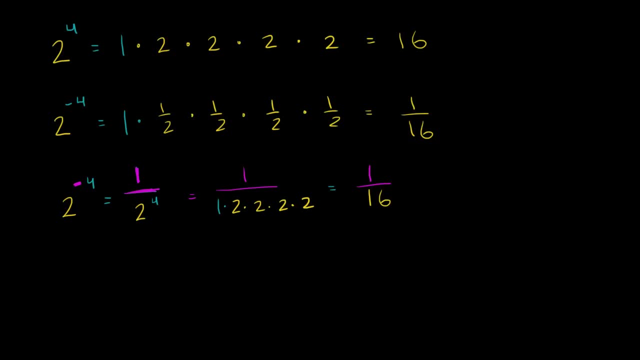 just so that we make sure things are clear to us. So let's try. 3 to the negative third power. So remember, whenever you see that negative, what my brain always does is say I need to take the reciprocal here. So this is going to be equal to: 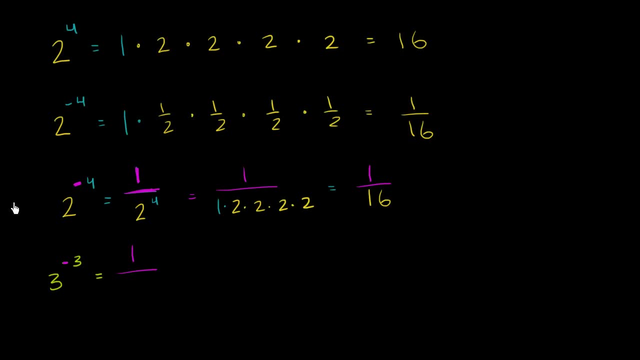 and I'm going to highlight the negative again. this is going to be 1 over 3 to the third power, which would be equal to well, 1 over 3 times 3, or you could say 1 over 3 times 3 times 3,. 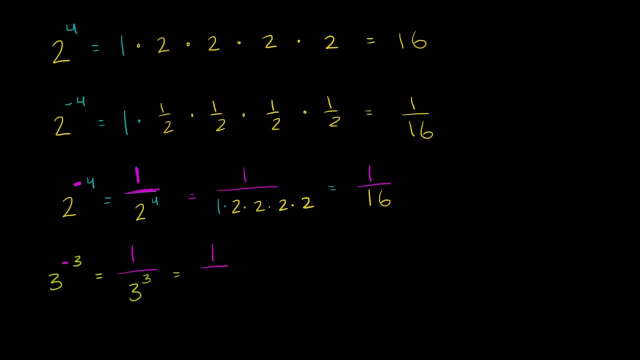 or 1 times 3 times 3 times 3 is going to be 27.. So this is going to be 1- 27th. Let's try another example. I'll do 2 or 3 more. So let's take a negative number to a negative exponent. 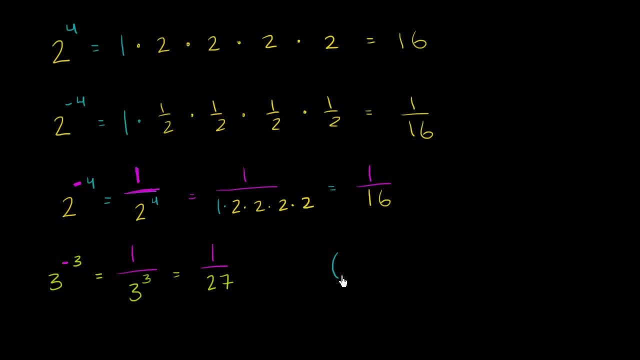 just to see if we can confuse ourselves. So let's take the number negative 4, and let's take it. I don't want my numbers to get too big too fast. So let's just take negative 2, and let's take it to the negative 3 power. 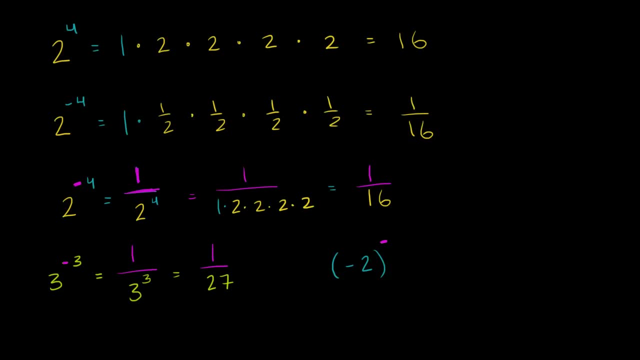 I want to make my negatives in magenta Negative 3 power. Negative 3 power. So at first this might be daunting. Do the negatives, cancel, And that'll just be the remnants in your brain that are trying to think of multiplying negatives. 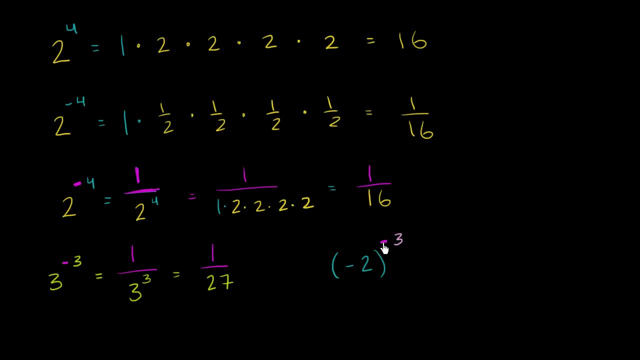 Do not apply that here. Remember you see a negative exponent that just means the reciprocal of the positive exponent, So 1 over negative, 2 to the third power, to the positive third power, And this is equal to. this is equal to: 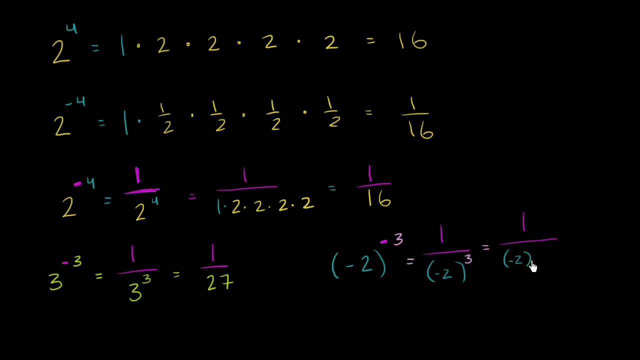 1 over negative, 2, negative 2 times negative, 2, times negative 2, times negative 2, or you could view it as 1 times negative, 2, times negative, 2, times negative 2,, which is going to give you 1 over negative 8,. 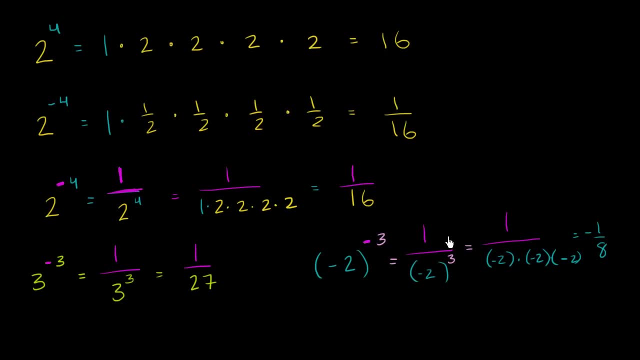 or negative 1 eighths. Let me scroll over a little bit, I don't want to have to start squinching things. So this is equal to negative 1 eighth. Let's do one more example, just in an attempt to confuse ourselves. 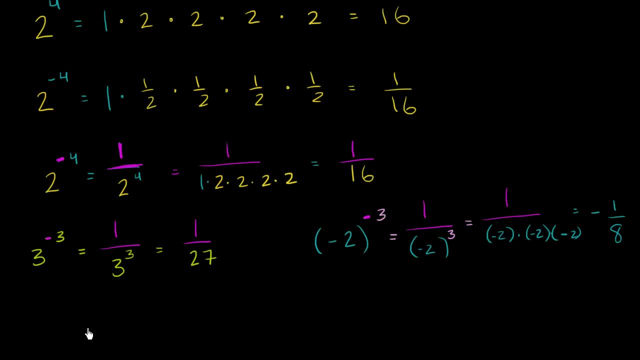 Let's take, let's take, I don't know. let's take 5 eighths and raise this to the negative negative 2 power. Negative 2 power. So once again this negative. oh, I got a fraction. 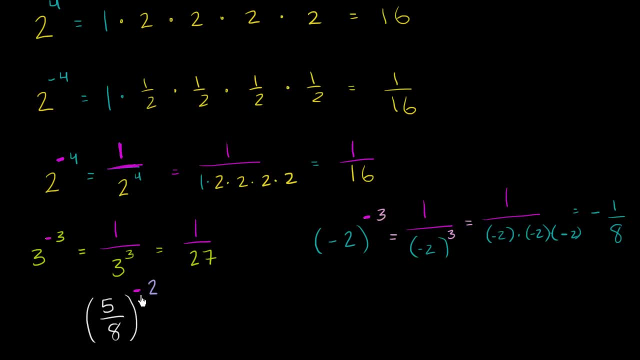 there's a negative here, Remember. this just means 1 over 5 eighths to the second power, So this is just going to be the same thing as 1 over as 1 over 5 eighths. 1 over 5 eighths, squared. 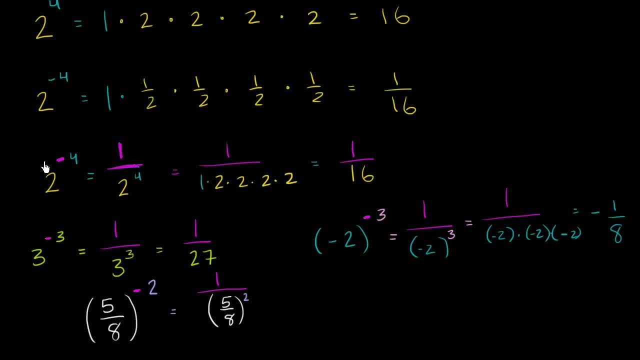 1 over 5 eighths squared, which is going to be the same thing. which is going to be the same thing, So this is going to be equal to- I'm trying to color code it- 1 over 5 eighths times 5 eighths. 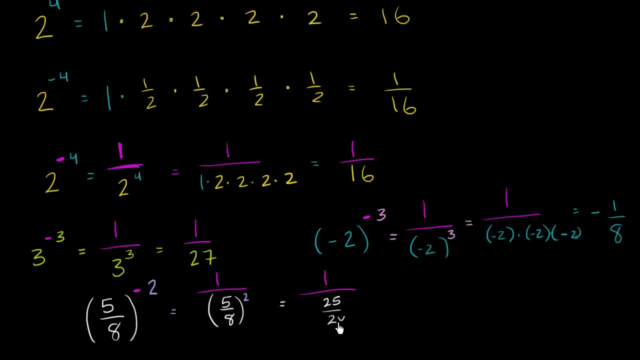 which is 25 over 60, 25 over 64.. 1 over 25 over 64 is going to be 64 over 25.. So another way to think about it is you're going to take the reciprocal of this and raise it. 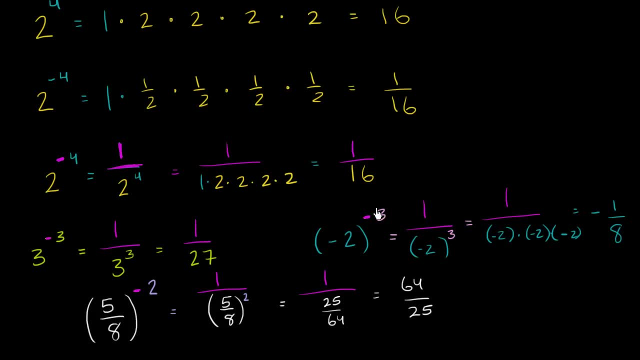 and raise it to the positive exponent. So another way you could have thought about this, another way you could have thought about this, is 5 eighths to the negative 2 power. Let me just take the reciprocal of this 8 fifths. 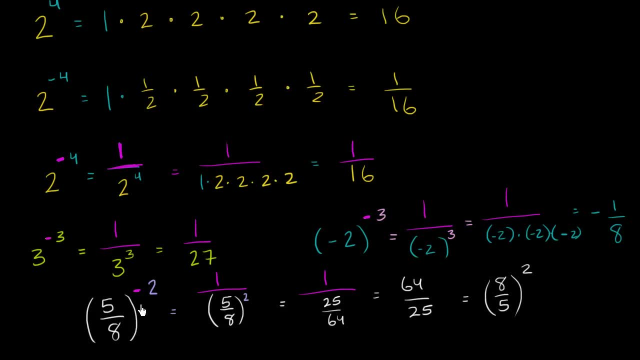 and raise it to the positive 2 power. So all of these statements are equivalent. And that would have applied even when you are dealing with non-fractions as your base right over here. So 2, you could say, well, this is going to be the same thing. 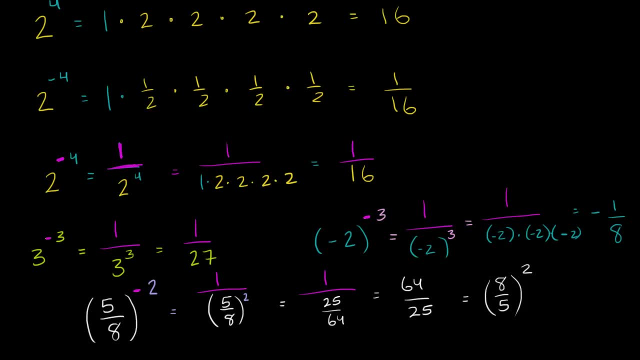 2 to the negative. 4 is going to be the same thing as taking my reciprocal. so this is going to be the same thing as taking the reciprocal of 2, which is 1 over 2, and raising it to the positive.